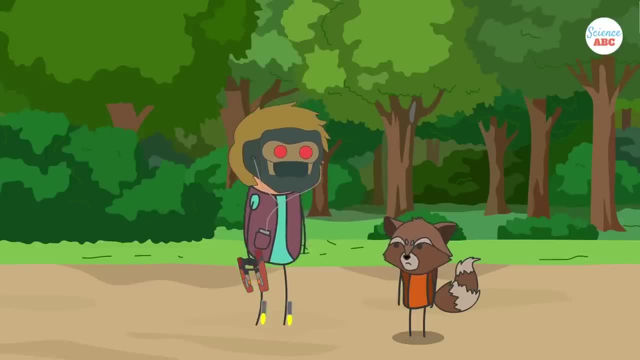 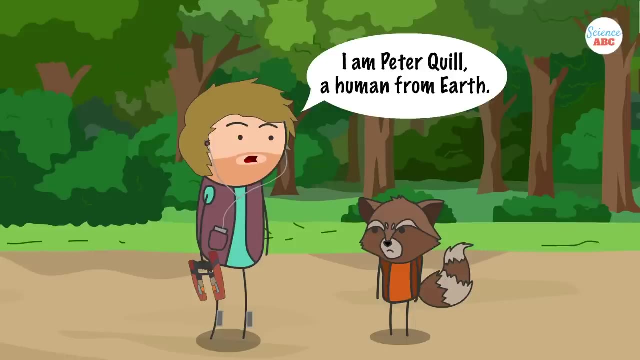 Now, let's assume, an anthropomorphic raccoon from another planet asks you the same question. What would you say then? Perhaps I am Peter Quill, a human from Earth. In this case, you specified three levels of identity. Your answer is one. 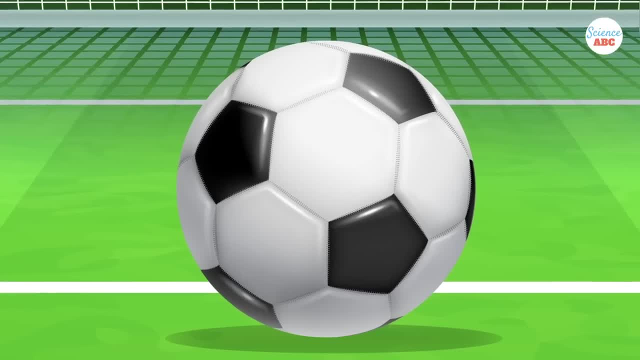 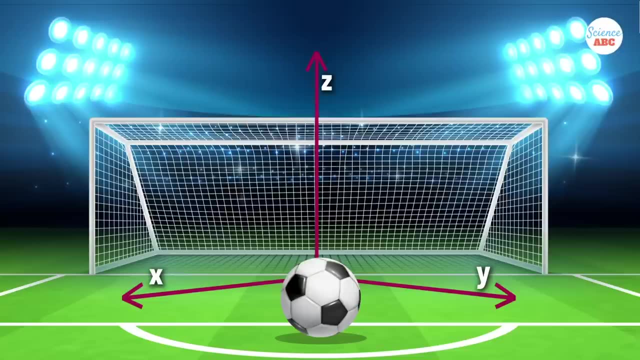 specified 3 levels of identification. Similarly, in a 3D space, x, y and z coordinates are used to specify an object's exact location, as no two objects can have the same x, y and z coordinates. If you consider a 4-dimensional space with time t as an additional dimension. 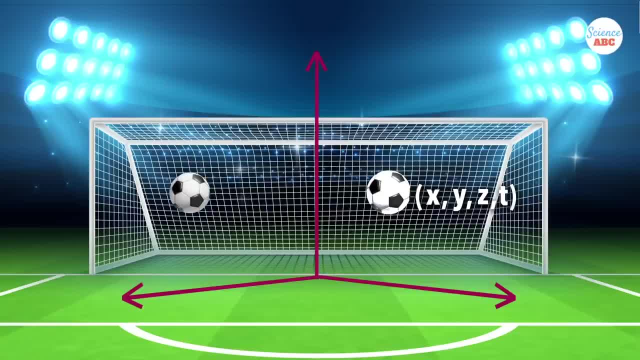 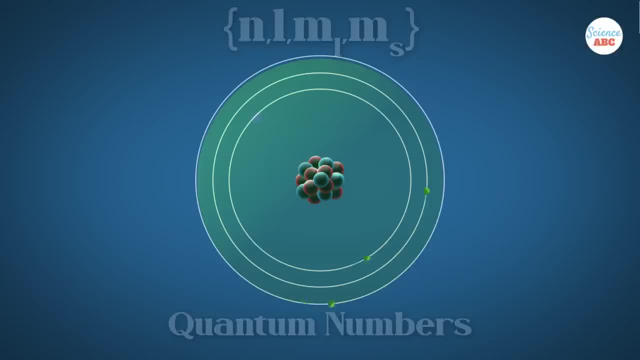 then no two particles can have the same 4 coordinates. In the same way, an electron has 4 levels of identification consisting of 4 quantum numbers. Every electron within an atom has a unique set of quantum numbers. No two electrons can share the same combination. 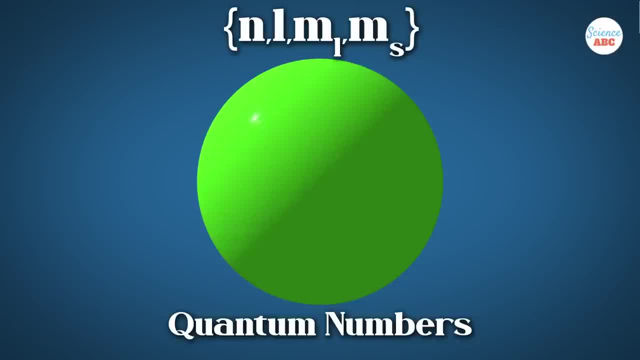 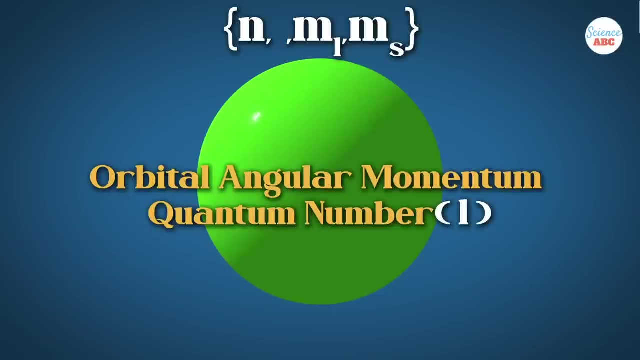 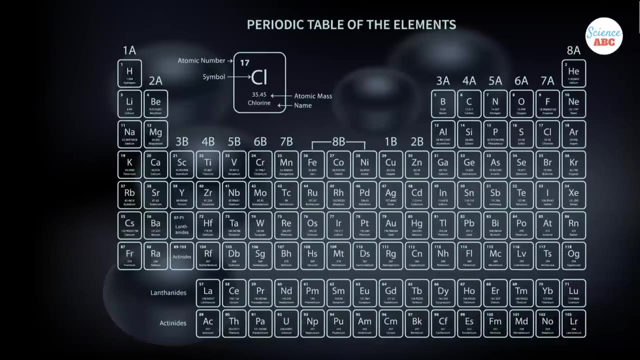 of 4 quantum numbers. Electrons can be identified using these 4 quantum numbers, which are called the principal quantum number: the orbital angular momentum quantum number, the magnetic quantum number and the electron spin quantum number. All of these quantum numbers are called the principal quantum number, the orbital angular. 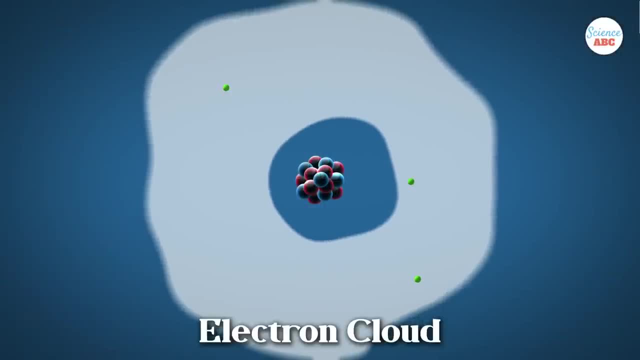 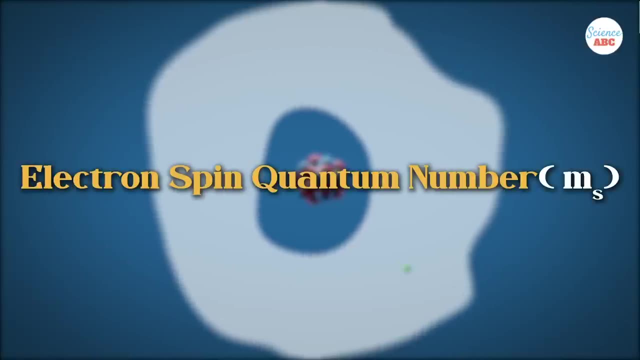 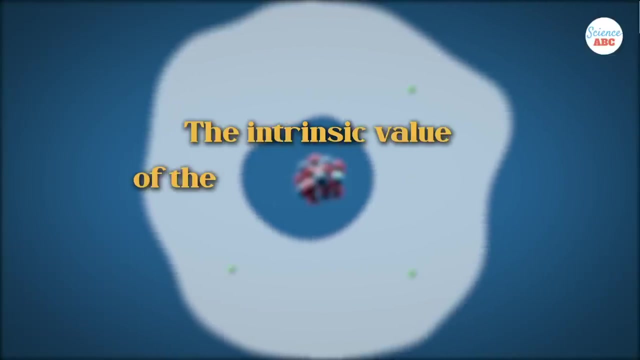 momentum quantum number, as they help determine the electron configuration of an atom and the probable location of electrons within that atom. However, for the scope of this video, we're only going to talk about the electron spin quantum number. The definition of spin is the intrinsic value of the angular momentum of a fundamental particle, An electron. 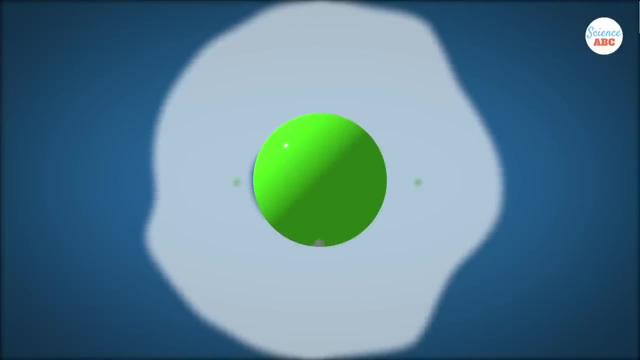 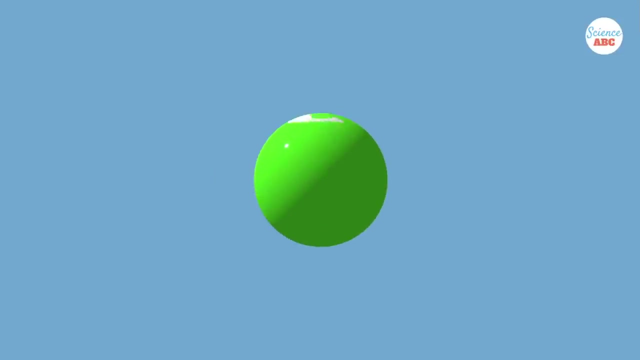 can either have a positive spin, called spin up, or a downward spin, called spin down. This is where things get bizarre. When we say an electron has a positive spin or a negative spin, it doesn't mean that the electron is actually spinning, Although it does have angular momentum and proper magnetic. 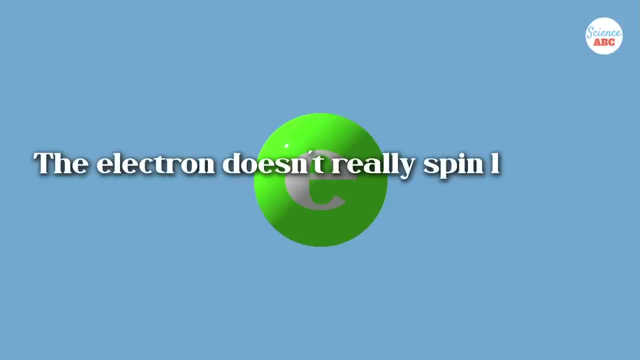 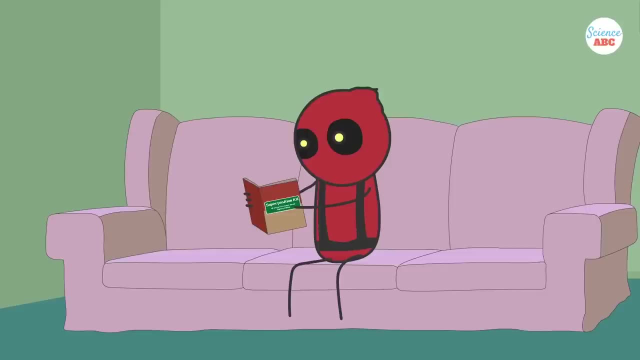 orientation. it's not exactly spinning. It may actually exist in a state of superposition, when it has both a negative and positive spin. You may find the idea of superposition confusing, because this doesn't seem to go along with our perception of the real world. To help, 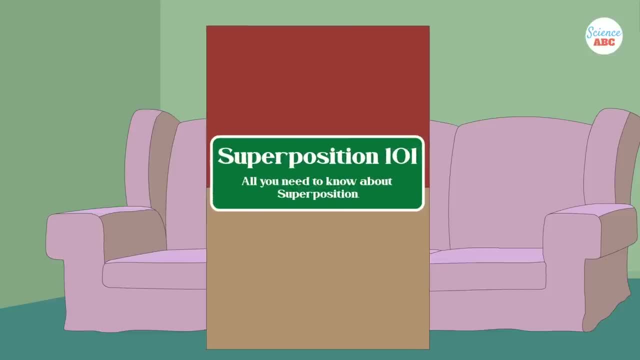 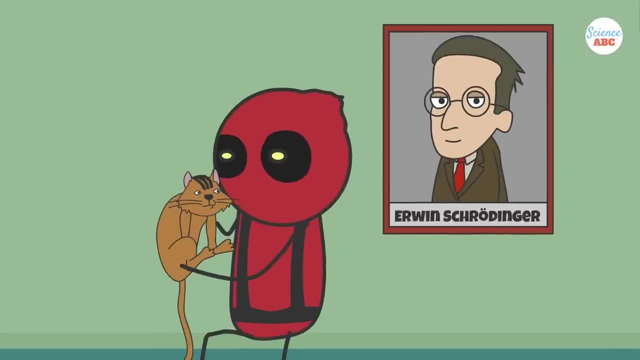 explain this a bit better, I'm going to use the term superposition. Superposition is a term that is used to describe a cat that is in a state of superposition. You might have heard of Schrodinger's cat. This is a famous thought experiment devised by Austrian-Irish. 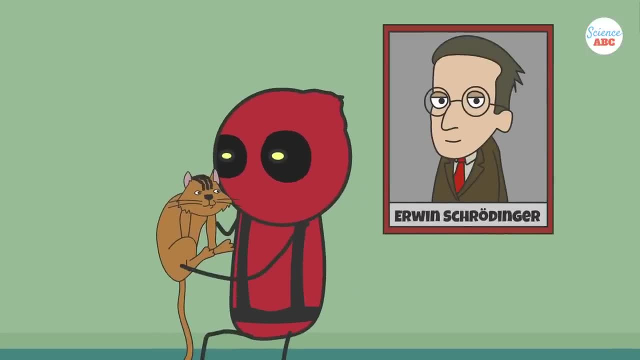 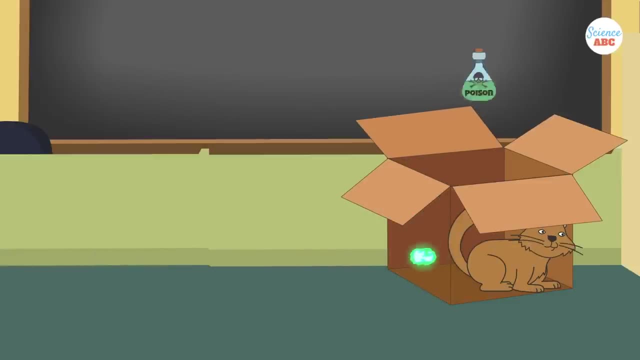 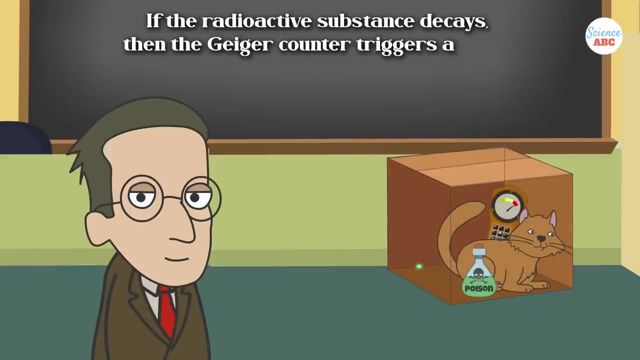 physicist Erwin Schrodinger. It goes something like this: Imagine that you put a cat inside an opaque, soundproof box along with a radioactive substance, a vial of poison and a Geiger counter. If the radioactive substance decays, then the Geiger counter triggers a setup that 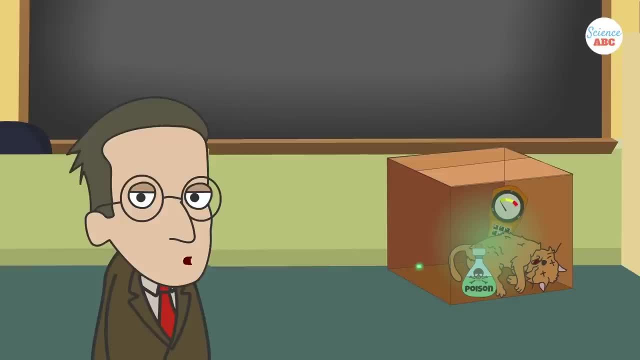 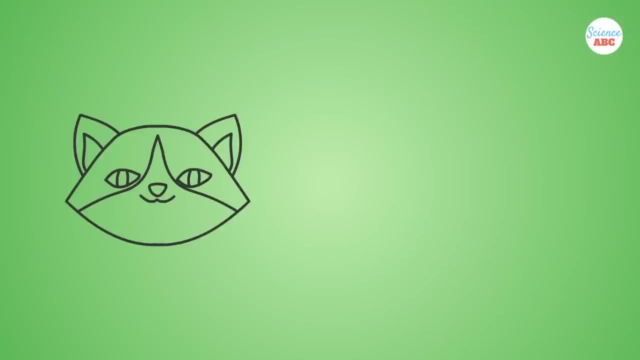 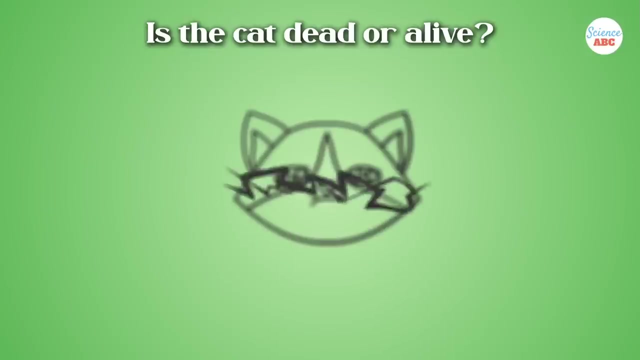 releases the poison, thus killing the cat. However, the decay of the substance is a random process, so there's no way to predict when it will happen, And that is why, before opening the box, you can say that the cat is in a superposition of being both alive and dead at the same time. 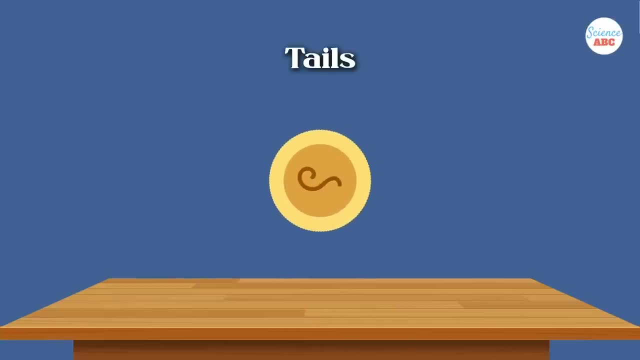 In the same way, when a coin spins on a flat surface, it's in a state of superposition between its two faces, heads and tails. Similarly, electrons in their natural state exist as a superposition of both up and down superposition. The source of superposition can be the mind's. 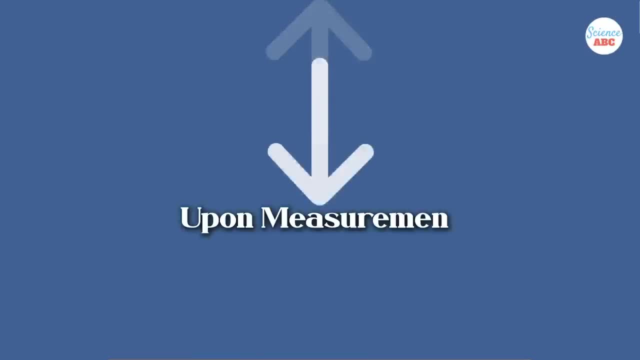 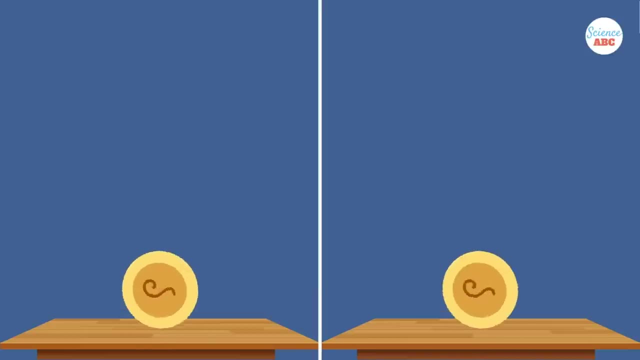 down spin. Only when measured do they give a definite value of up or down, which in technical terms, is referred to as the collapse of the wave function. In quantum mechanics, wave function collapse occurs when a wave function which was initially in a superposition of a few states. 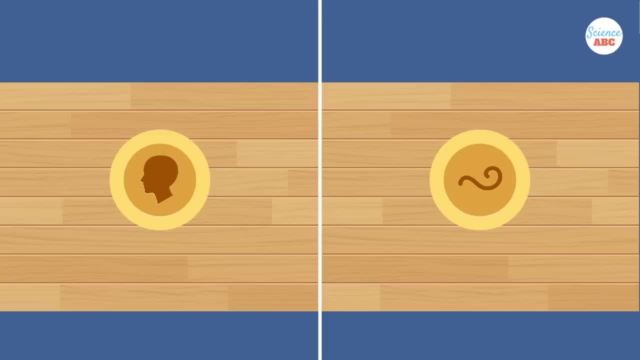 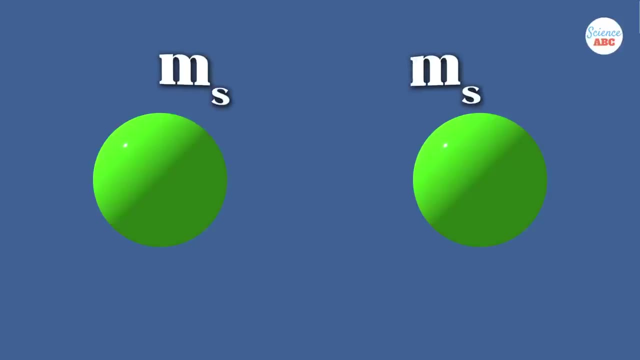 reduces to a single state due to interaction with the external world. When a pair of electrons are generated, interact or share spatial proximity, their spin states can get entangled, which is what scientists call the quantum entanglement of electrons. Once the electrons are entangled, 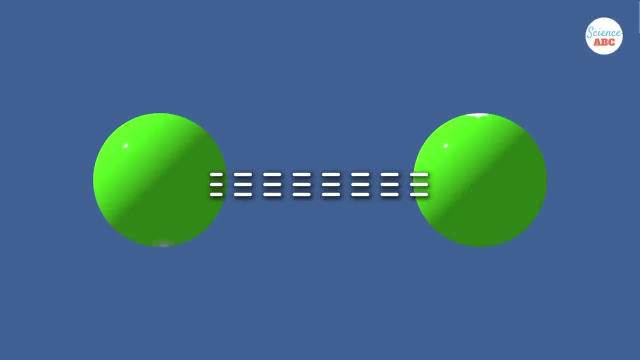 the two electrons can only have opposite spins. That is, if one is measured to have up spin, the second immediately becomes down spin. Now we know that the two electrons unmeasured do not have a single spin, but a superposition of both up and down spin. If we were to separate 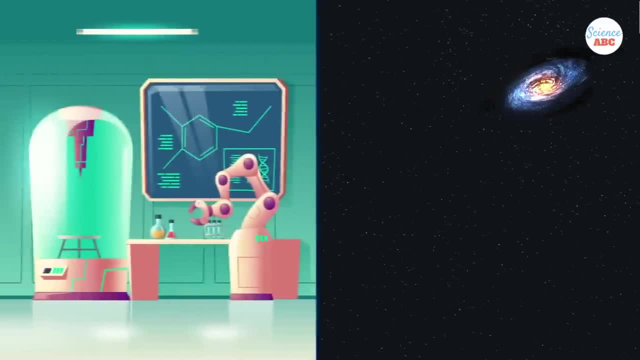 the two electrons arbitrarily far, say we put one in a physics lab on Earth and the other one in a physics lab on Earth, we would have a superposition of both up and down spin In a different lab somewhere in the Andromeda galaxy and we measure the spin of the electron. 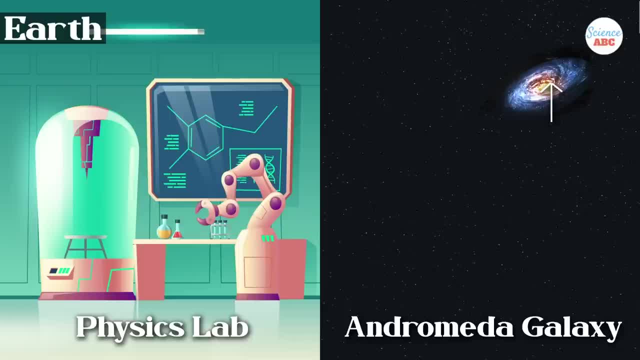 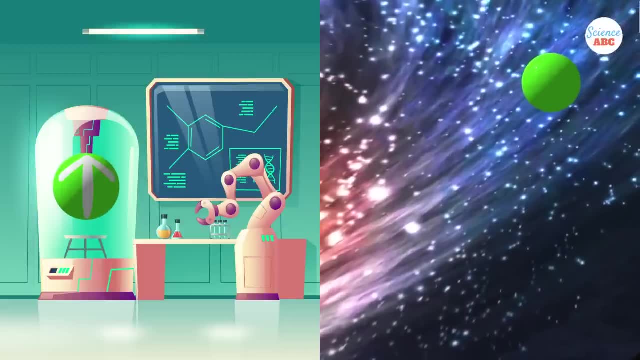 on Earth, we will immediately know the measurement of the one in the Andromeda galaxy. For example, if we measure the Earth electron to have up spin, we immediately know that the other electron has down spin. This information traveled instantaneously faster than the speed of light. 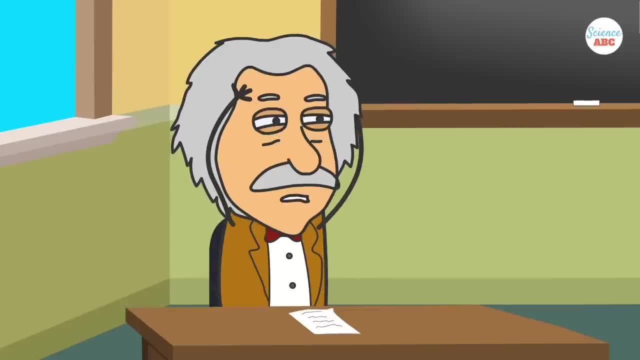 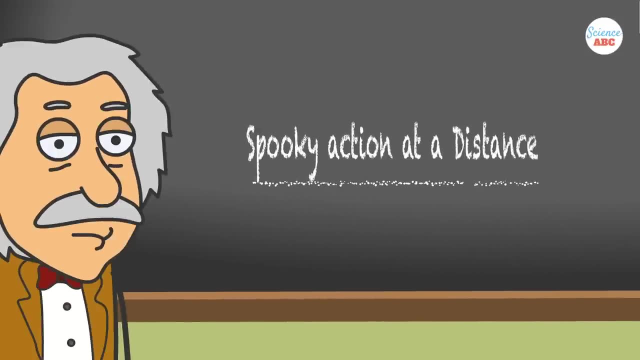 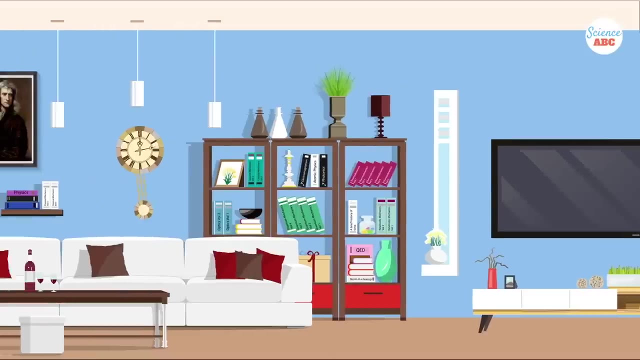 As one can imagine, this idea greatly bothered famous physicist Albert Einstein. It was such a disturbing realization, in fact, that he called this phenomenon spooky action at a distance. So how can this spooky action at a distance be useful to us? Well, let's start with one of the 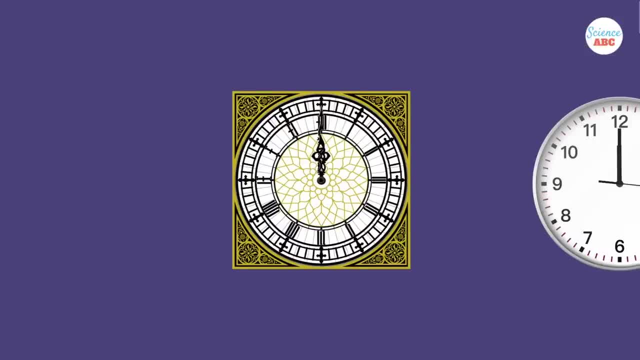 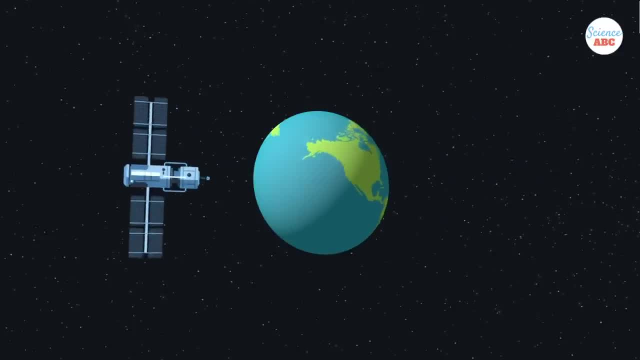 most common everyday objects, the clock. Having a common synchronized clock is very important in today's world. They keep things in line, like stock markets and GPS systems. Today we have extremely precise clocks, known as atomic clocks, The quantum logic clock, which is the clock that 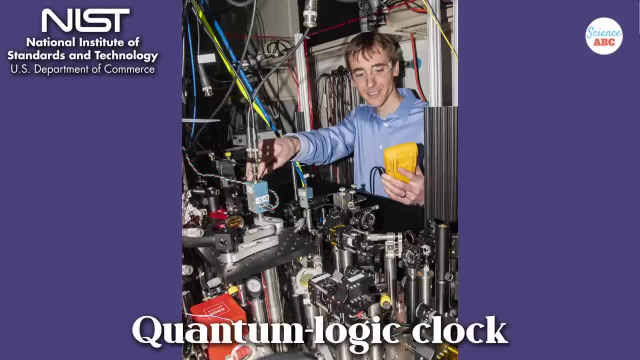 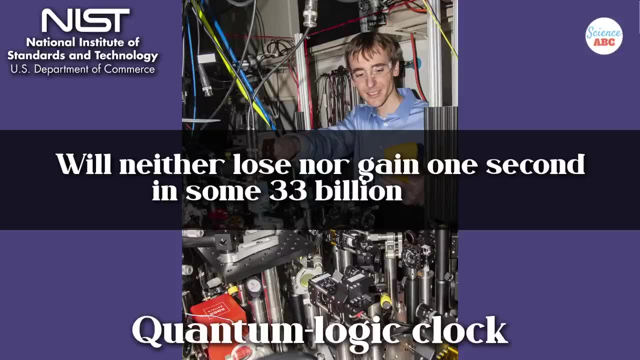 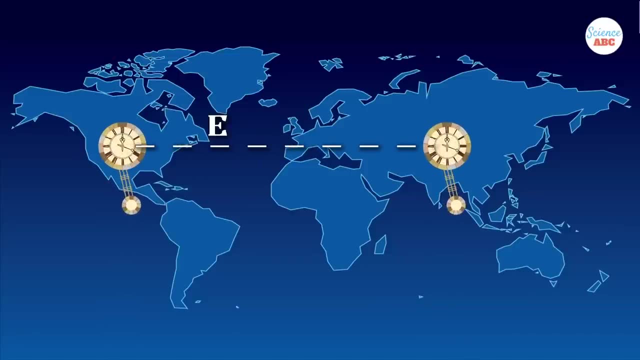 the US National Institute of Standards and Technology, NIST, in Colorado, will neither lose nor gain one second in some 33 billion years. Entangled atomic systems would not be preoccupied with local differences and would instead solely measure the passage of time, effectively bringing 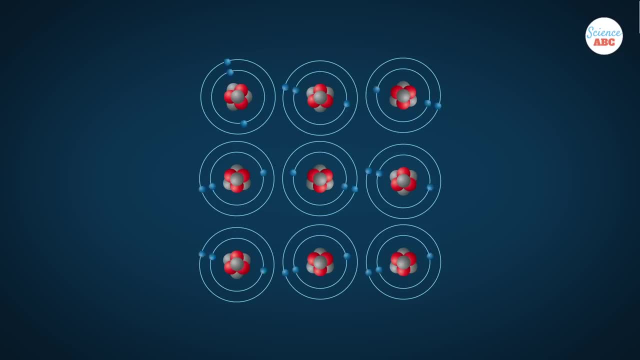 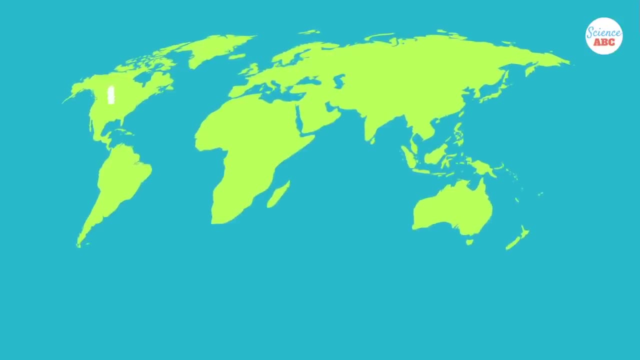 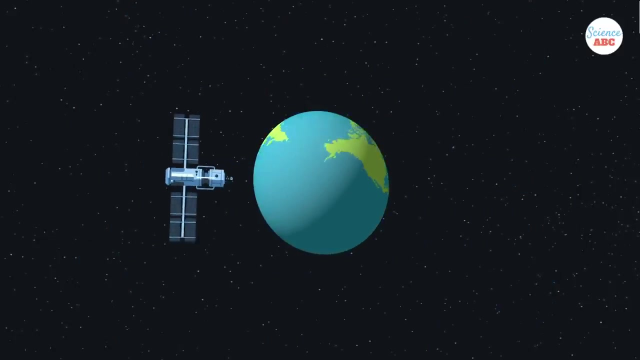 them together as a single pendulum. That means adding 100 times more atoms into an entangled clock would make it 100 times more precise. Entangled clocks could even be linked to form a worldwide network that would measure time independent of location, vastly expanding the technology of GPS systems and telecommunication. 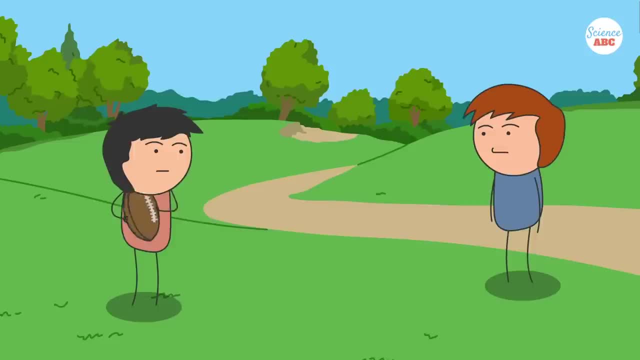 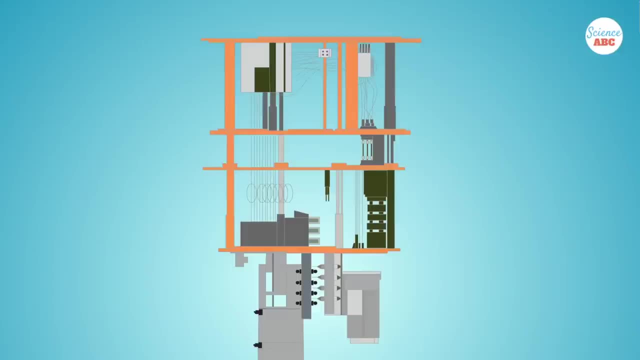 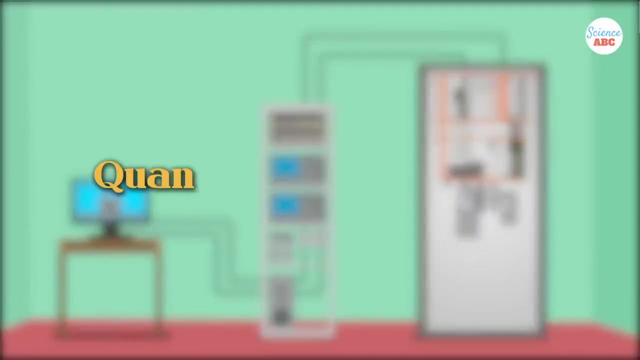 Then, of course, there's quantum cryptography. As a kid, did you ever make up a secret code, language that only you and your best friend could understand? Imagine that, but with the key to cracking the code being randomly polarized photons entangled with each other. That is quantum cryptography. 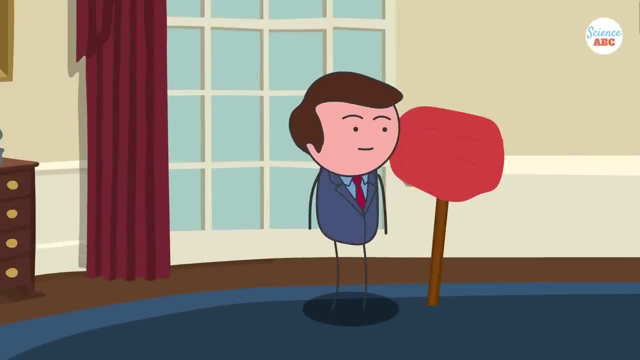 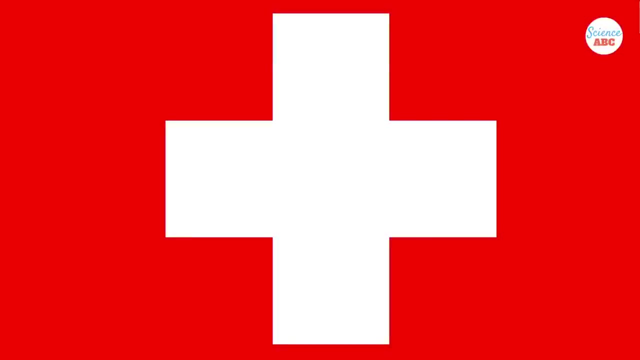 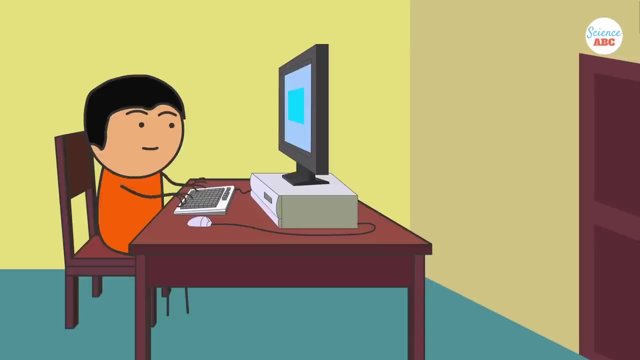 Today, some tech companies use QKD- quantum key distribution- to design ultra-secure networks. In 2007,, Switzerland tried out an iD Quantique product to provide a tamper-proof voting system during an election. This system promises to be highly secure because if the photons are entangled,